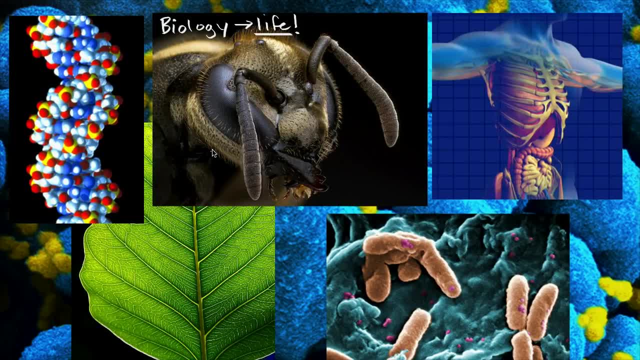 And we get the complexity of living things. And you might be saying: well, what makes something living? Well, living things convert energy from one form to another. They use that energy to grow. They use that energy to change, And I guess growth is a form of change. 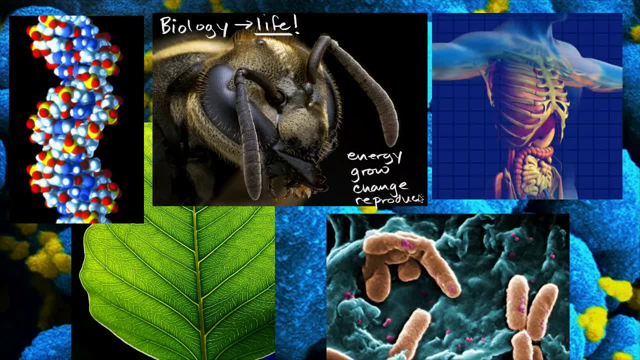 They use that energy to reproduce, And these are all in and of themselves, fascinating questions. How do they do this? You know, we look around us, how do we eat a muffin, And how does that allow us to move around? 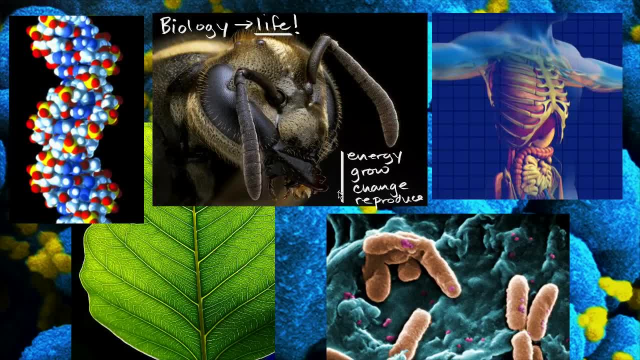 and think and do all the things we do. Where did the energy from that muffin come from? How are we similar to a plant or an insect? And we are eerily or strangely similar to these things. We actually have a lot more in common. 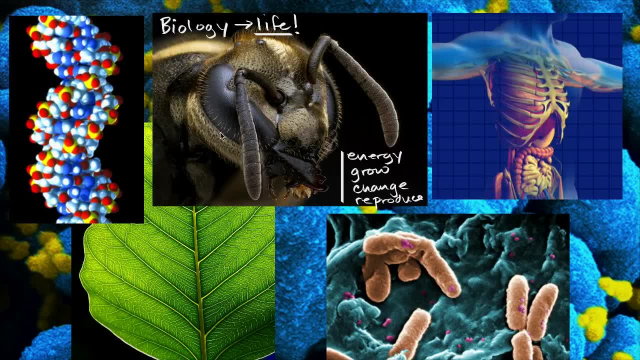 with that tree outside your window or that insect, that bee that might be buzzing around. Then you realize, even with the bacteria, that you can only even see at a microscopic level. In fact, we have so much bacteria as part of what makes us us. 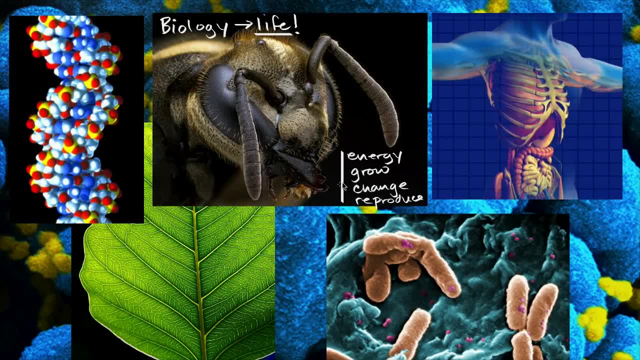 So these are fascinating questions. How do we, how did life even emerge? And so, over the course of what you see in biology on Khan Academy, we're going to answer these fundamental, fascinating questions. We're gonna think about things like energy and the role of energy in life. 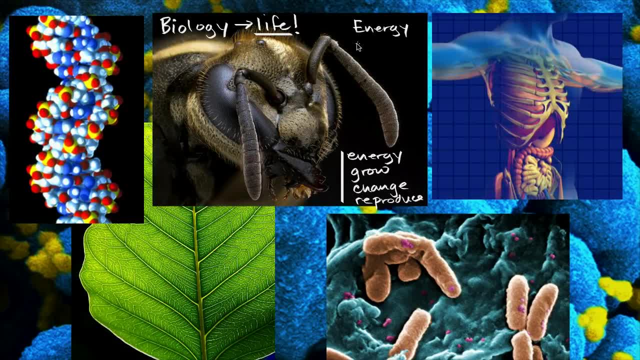 We're going to think about important molecules in biology and perhaps most importantly, DNA and its role in reproduction and containing information, And we're going to study cells, which are the basic building block of life. And, as we'll see, even though we view cells, 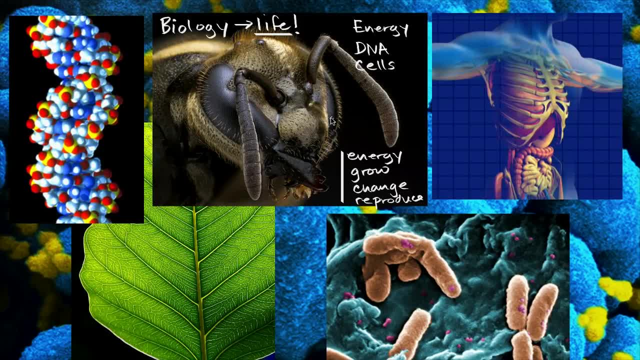 as these super, super small, small things. cells in and of themselves are incredibly complex And if you compare them to an atomic scale, they're not that large. In fact, this entire, this blue background that I have there, that's the surface of an immune cell. 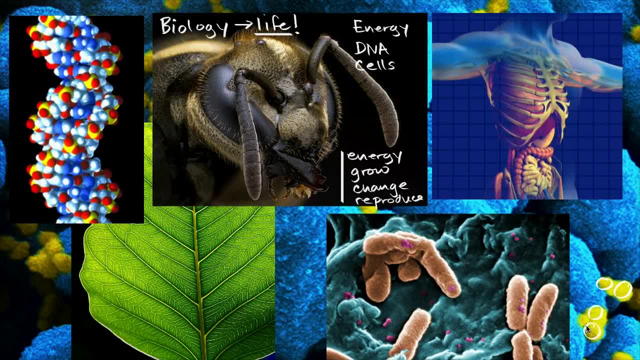 And what you see here emerging from it, these little yellow things. these are HIV viruses emerging from an immune cell. So even though you imagine cells as these very, very small, microscopic things, there's incredible complexity, even viruses. Viruses are one of these fascinating things.